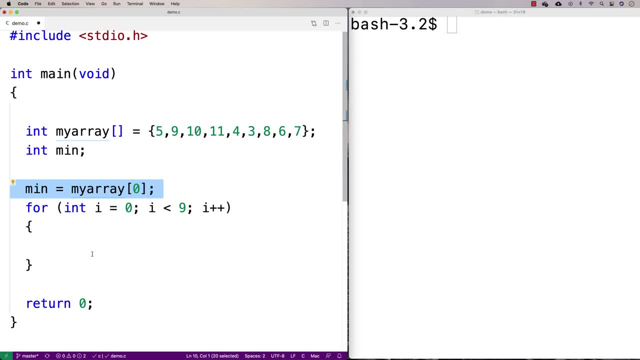 is less than our current minimum number and if it is, we're going to make that the new minimum number. so we're going to say here: if min- or- we're sorry- we're going to say if my array at i is less than min, then make min equal to my array at i, make that the new minimum number. 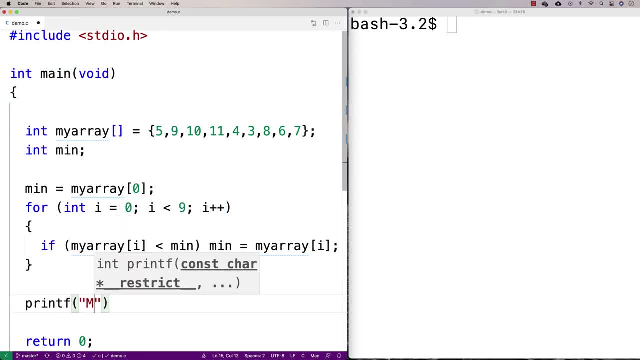 and then what we could do is we could then print out the minimum number at the end here, so we could say min minimum, min minimum say %d slash n, and we'll print out min. And so if we run this here we'll get, if the minimum number 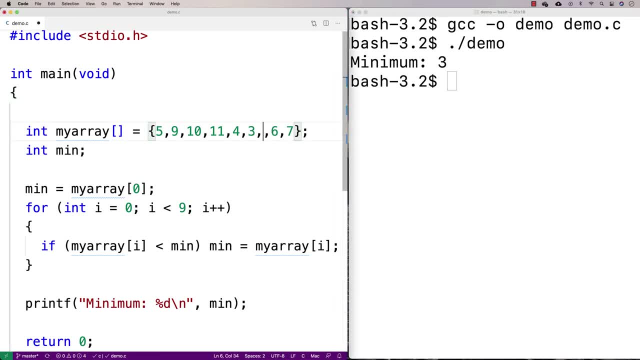 is three, and that makes sense based on what we've got here. If I change like eight to one, then recompile it and run it again. we find the new minimum number is one, and so it appears to be working. So now there's a couple things we could do to make this better. So one thing is: 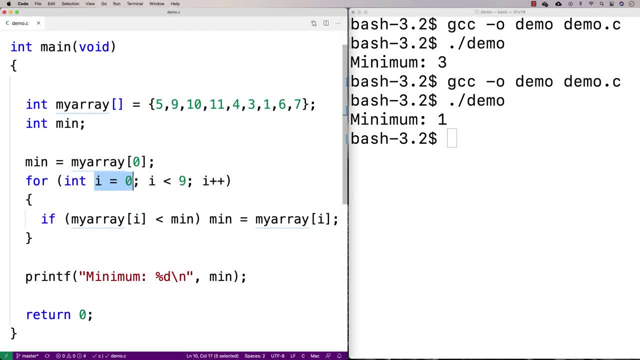 I started off my loop going from zero until nine, incrementing by one, and I did that because nine is the length of the array here. Now, one thing about this is that I don't really need to check zero, right, I don't really need to check that my array at zero is less than min, because you know if that's. 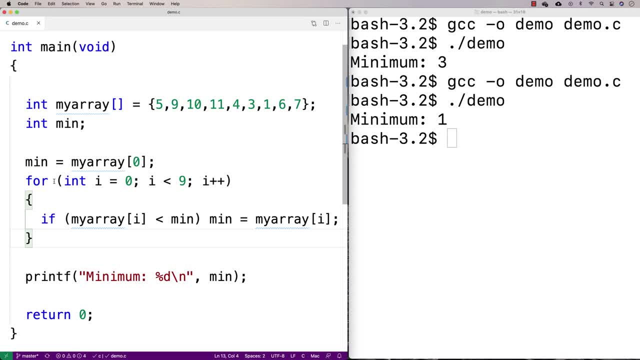 the case, then it doesn't make any sense because we just set min to my array at zero, right? This can't really be the case. So I'm going to check my array at zero and I'm going to check my array at zero. So in this case, that for when i is zero, that my array at zero is going to be less than min. 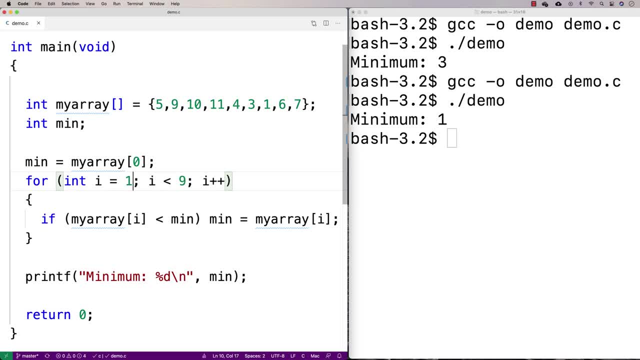 because we just set it to that, So I can actually start i off at one, and it's going to be just as accurate as it was before. It'll find the same minimum number, no matter what I can make this zero here, for example, and it'll still work. It'll still find the correct minimum number. 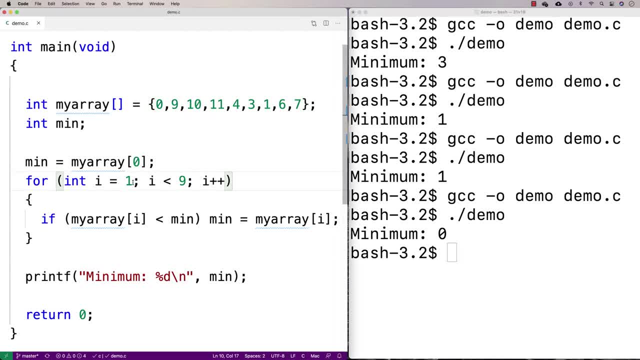 It'll be zero now, right? So I don't really need to check that first value in the array because I'm already starting with that as my assumed minimum Number and I'm checking all of the minimum numbers as we go and and you can see how the 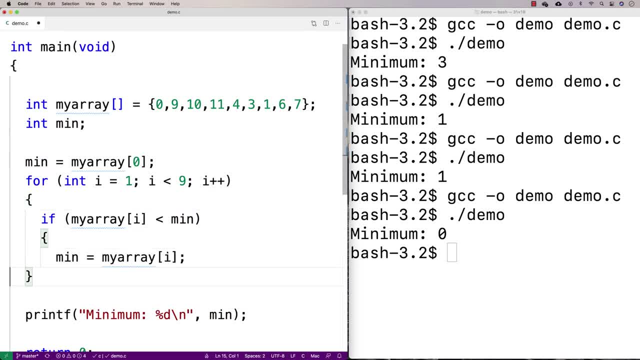 algorithm works Like if ever you're coding and you're trying to figure out, like, how does my algorithm work, One thing you can always do is just throw in a ton of printfs. So just throw in lots of printfs to figure out how something's going to work. So with this here what we could. 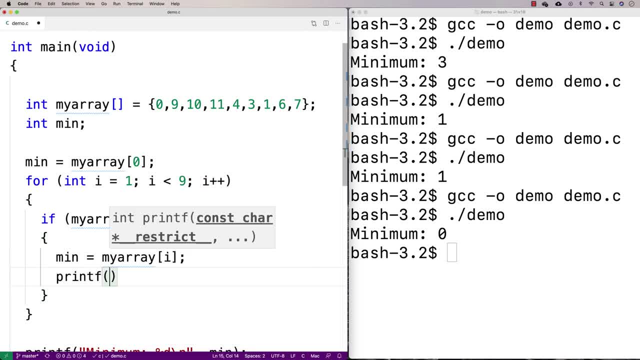 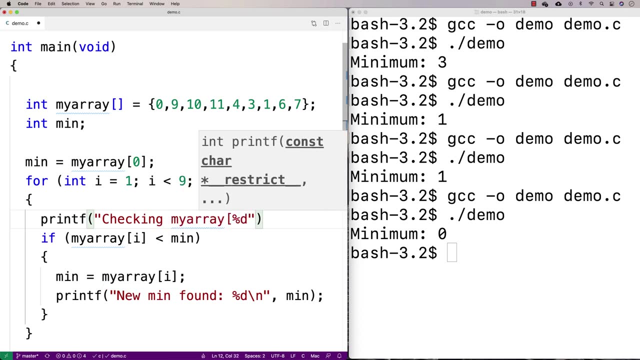 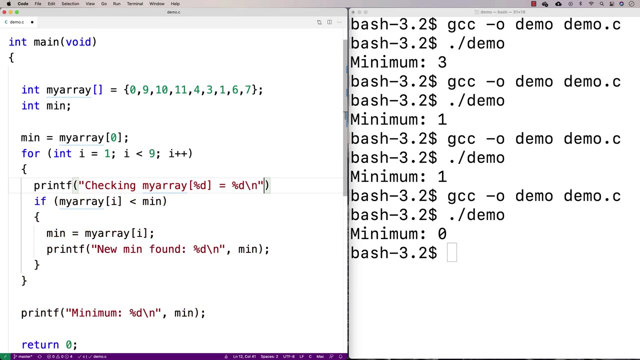 do is we could throw in a printf and we could say: like printf and we'll say: new min found percent d and we'll print out min. And here we'll printf and we'll say checking and we'll say printf and we'll say: maybe my array percent d is equal to percent d, and then we'll print out i and we'll print out. 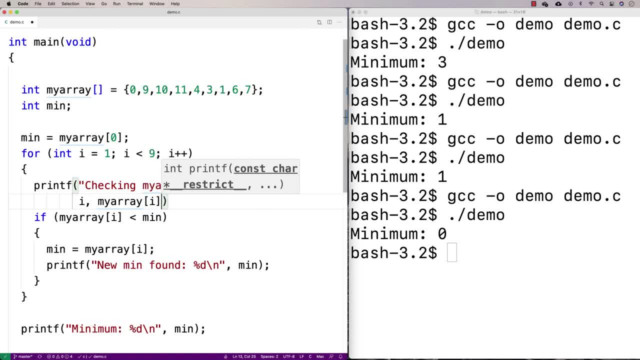 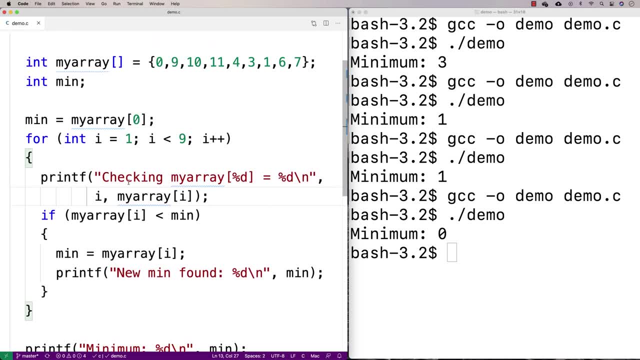 my array. So we'll print out i and we'll print out my array at i And what this will do here. maybe I can make it bigger again. Yeah, I can make it bigger again. We'll make it so that we print out what my array at i is and we're going to print out whenever we 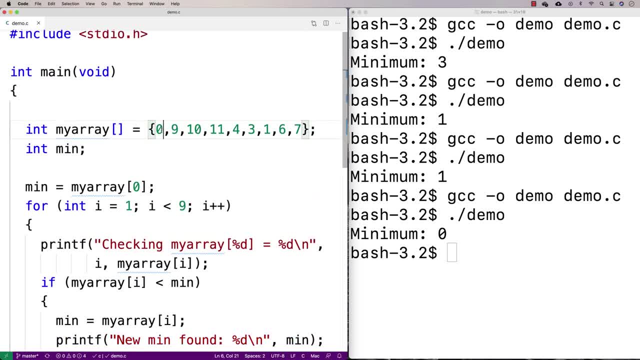 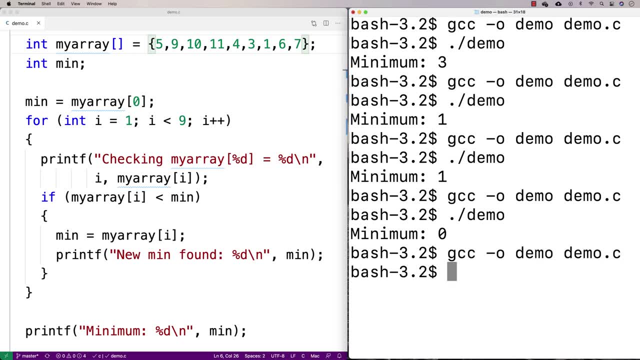 find a new minimum And we'll. maybe we'll start with some new numbers here also. So I'll say here like five, and yeah, we'll do this, This should be okay. So let's just output this just to see what we get. So here we see, you know, checking my array. 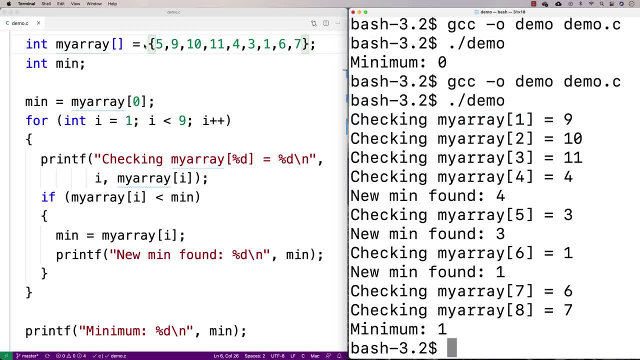 at one is nine. checking my array at two is ten. checking my array at three is eleven. and you can see that we're checking like nine, ten, eleven and so forth. We don't. we don't check the first one because we're skipping over it, because we already said that's. 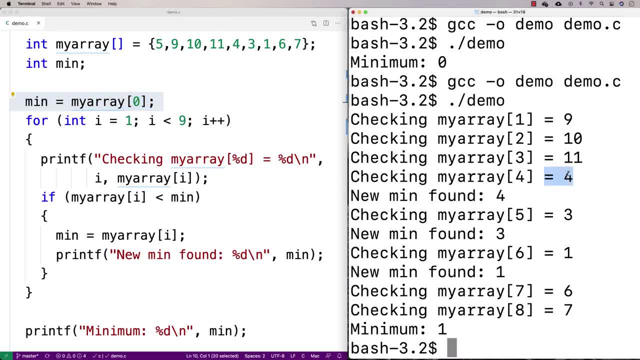 the minimum. And here, when we reach four, we find a new minimum. It says new min found. So we know that we've entered into this if statement here, right, And, and that's you know, letting us know this with this printf here, with this output here It's letting us know that we entered into this if. 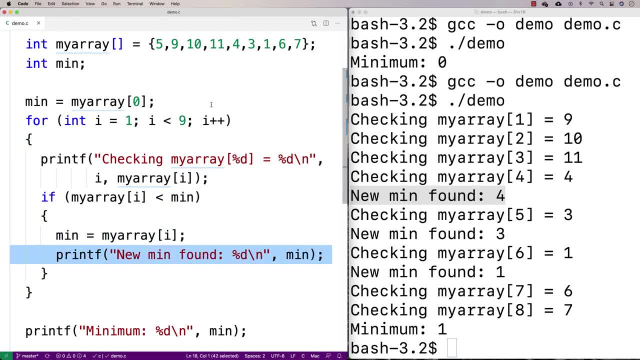 and we found a new minimum. And it makes sense that we found a new minimum when you know, my array at four is equal to four because we started off with five as the minimum. So four would be the first thing, that's less than it. And then we check my array at five, which is three. 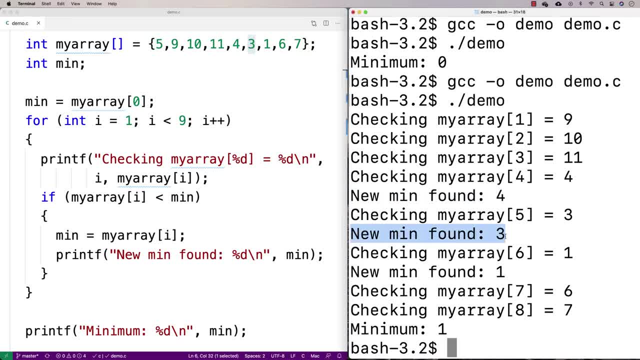 And that makes sense, that that would also be a new minimum because it's less than four. Then we check one and we- that makes sense, that would also be a new minimum, because one is less than three, and on and on right, And so, anytime you're, you're kind of trying to figure out how. 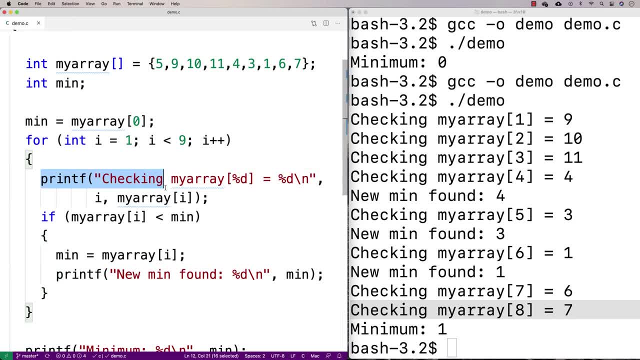 some kind of algorithm works or how your code works, throwing in printfs and just outputting your, your values that you're going through, say, in an array, or outputting you know what some if statement has identified. This can be a great way to help you figure out what's going on in your 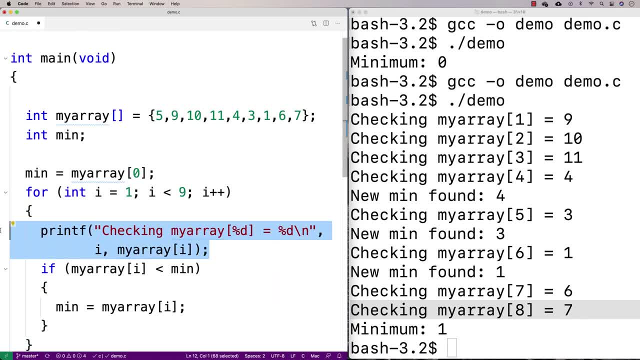 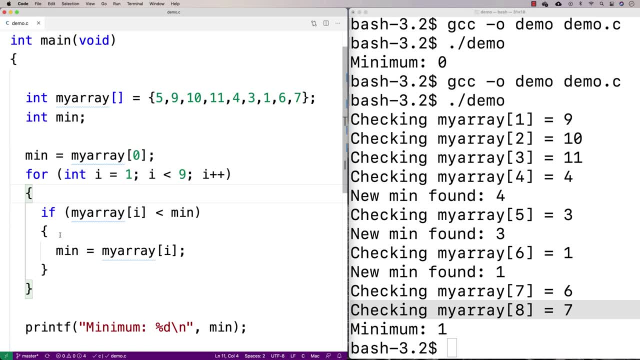 code. So okay, so we'll, we'll get rid of these things here now, because we're confident that we're going to get rid of these things right here Now. one thing we might want to do is we might want to put this inside a function, So that way we can call the function to find the minimum. 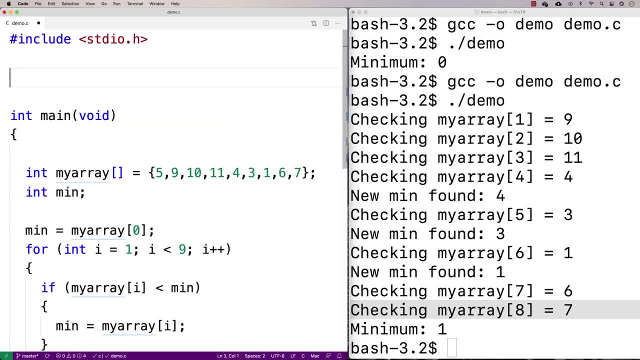 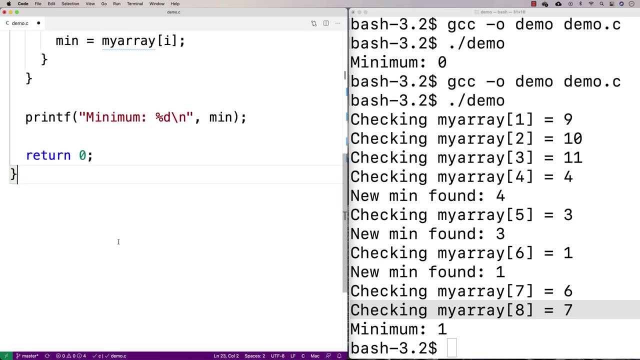 value whenever we want it. So if I want to do that, I'll put a. well, we'll put the function definition up here. I'm going to say find min and I'm going to say int array, and then I'm going to say int length, And then down here we'll make our function body look like this: 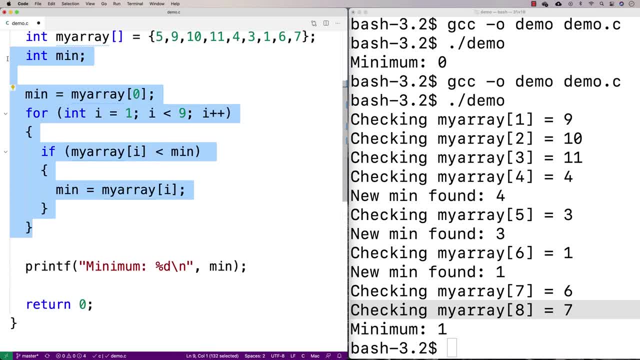 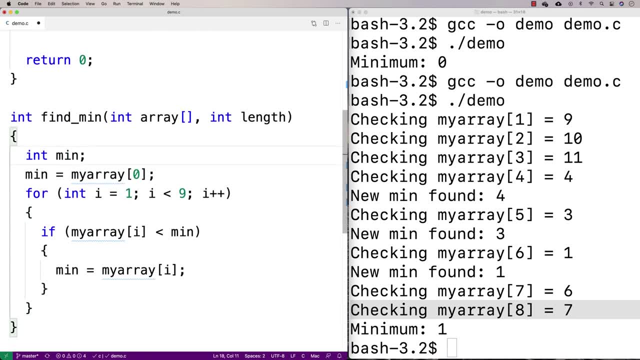 So what we're going to do is we're just going to take this logic here and we're going to put it inside the function, So that way we can kind of call this whenever we need it. So I can call find minimum for maybe different arrays and find the minimum for for each array, And I called it array here. 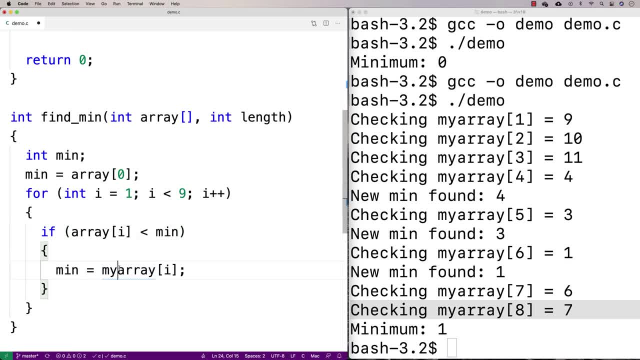 instead of my array. So I'm just going to change these to be array instead of my array, And then what we'll do is we'll return the minimum value here. So what I've got here now is a function, find min, that's going to take in an array as an argument and a integer length as an argument, And 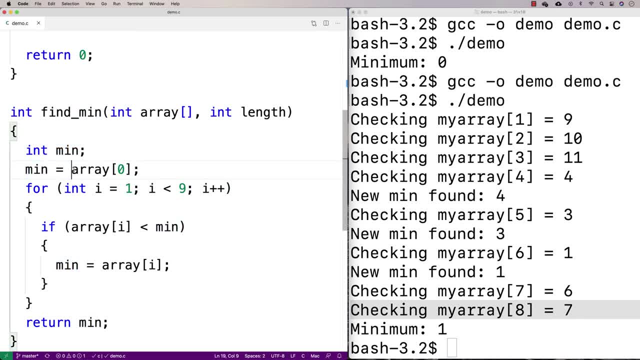 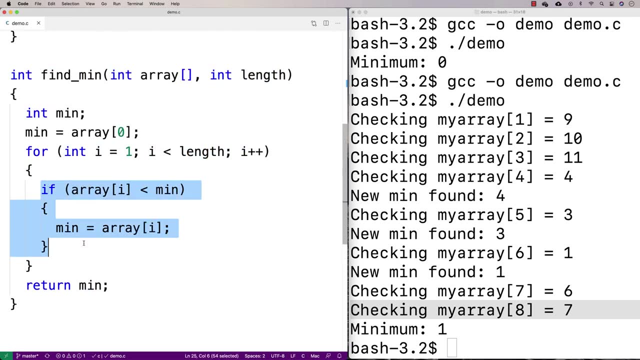 I'm going to set min equal to the first element, the array. again, It's going to loop from one until I'm going to say the length of the array, The length of the array, so I can give it arrays of different length, and it'll still still find the minimum value And it's going to keep doing. 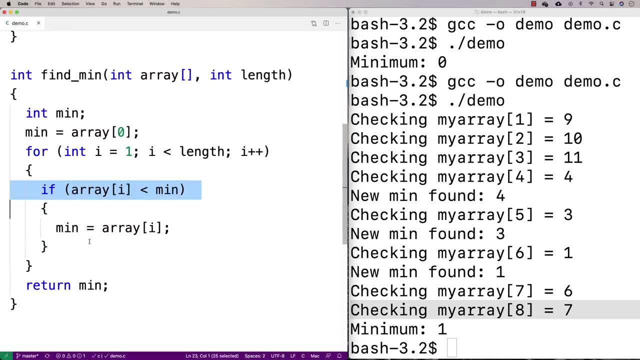 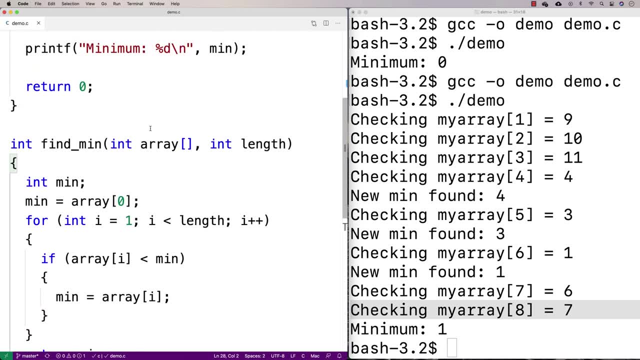 our algorithm where we just keep on checking the values in the array. If we find a new minimum, make that the new minimum and we're going to return the minimum. So I've got this function here. now that should be pretty generalizable. now I should be able to call it for different arrays. 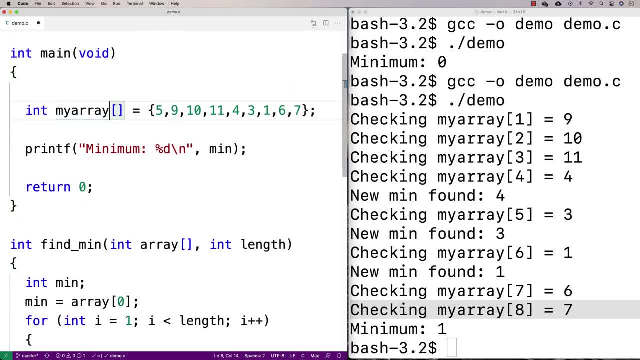 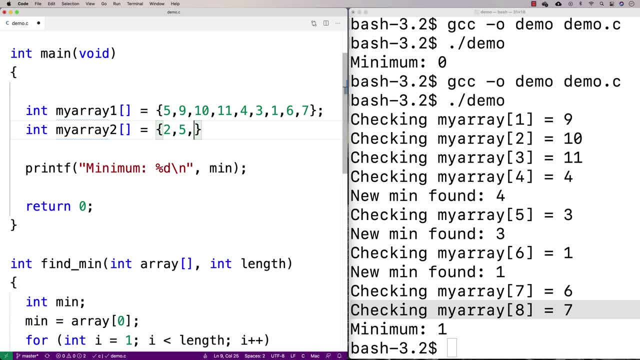 What I could do is we could have my array one and then I'll make my array two And I'll make this a different length. I'll say two, five, nine. two, five, four, three And I'll say maybe zero. 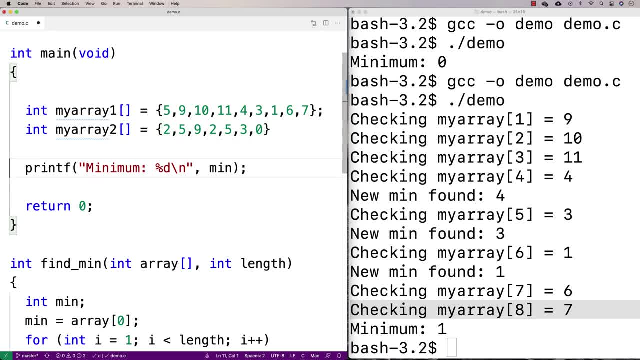 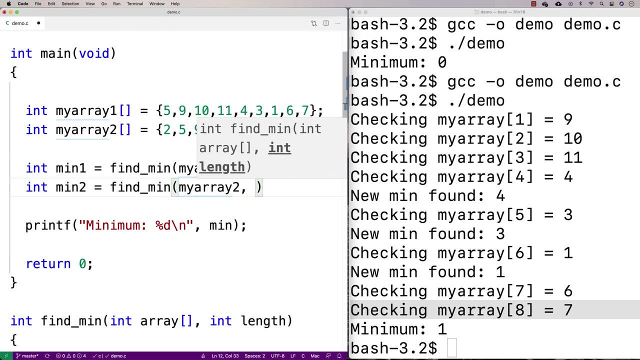 here at the end And I could say: maybe we'll find the minimum for both now. So we'll say int min one is equal to find min, and we'll call the function with my array one and we'll give it the length nine. I could say int min two, We'll say find min, my array two And we'll give it length. What do we?